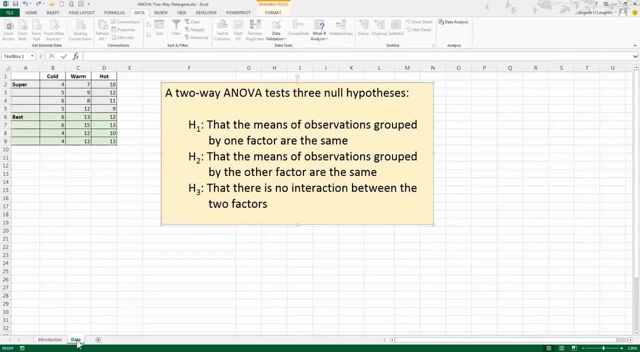 So in this design here our factor temperature has three levels and our brand has two. In a two-way ANOVA we set out three null hypotheses. Our first, H1, is that the means of observations grouped by one factor are the same. So in our example here this will be that: 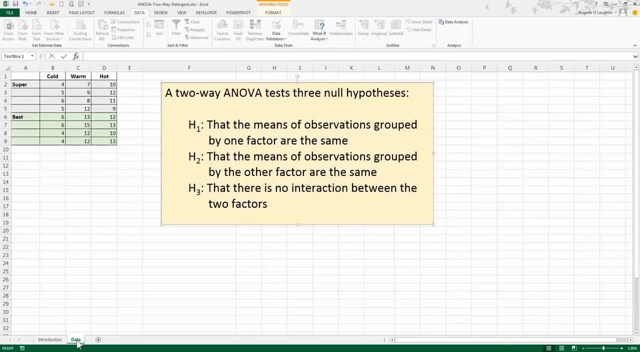 there's no difference between the means of the super and best brands. Our second hypothesis, H2, is that the means of observations grouped by the other factor are the same. In other words, we're testing here to see if there's a difference between the cold, warm and hot temperatures. 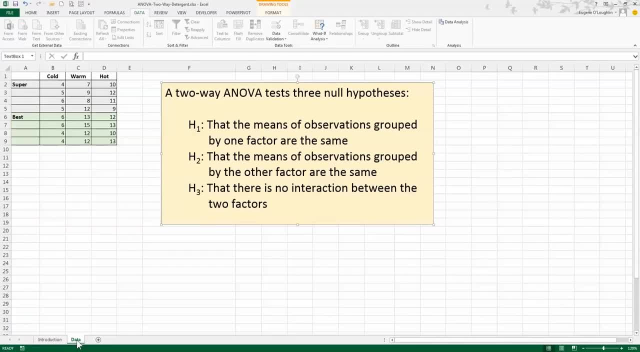 And our third hypothesis is all about the interaction between the factors. H3 is that there's no interaction between the two factors. In other words, the effect, for example, of temperature on dirt remove is not dependent on brand. So we're going to test for that, So just move the. 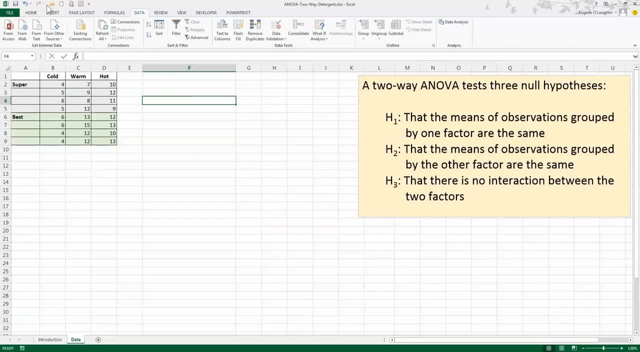 hypothesis over to the right hand side here. Now, when I'm conducting a two-way ANOVA, the ribbon I need first of all here is the data ribbon across the top of Excel And then over towards the right hand side on the analysis pane. I've got the data analysis tool pack option Now. 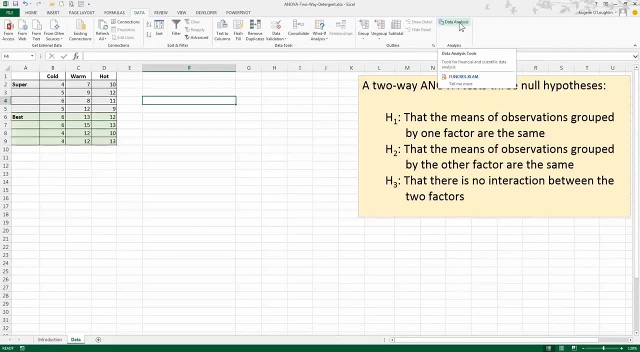 if you don't see this here, it means that you do not have this add-on installed in Excel. You'll need to add this in separately. So click on data analysis and this gives me our data analysis tool pack showing lots and lots of different statistics. The one that we need to use here is the ANOVA. 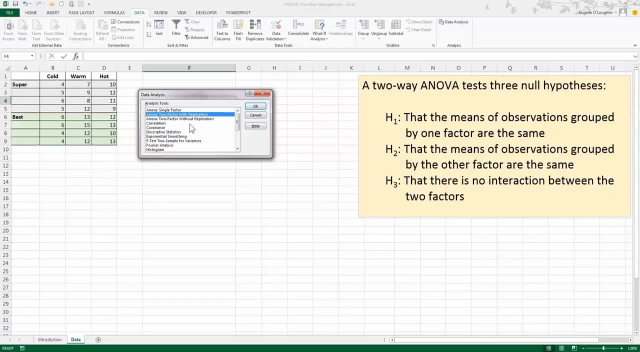 two-factor with replication, because we need to use the ANOVA two-factor with replication, So we're going to have more than one observation for each combination of our variables here. So select ANOVA two-factor with replication and click on OK. Now there are just a few things you need to input here. 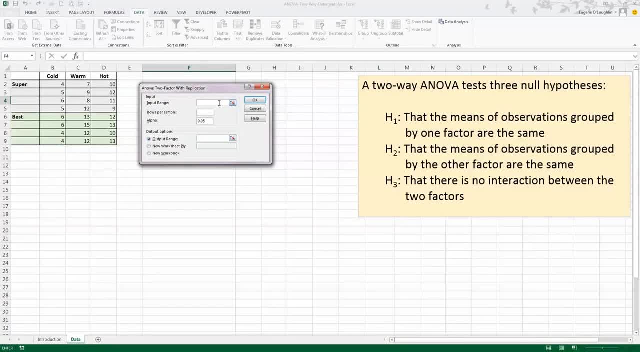 in the two-factor with replication window. First of all, you notice that there's only one input range. So that's fairly straightforward: Just select everything in your data. So it's important that your data must be laid out like this. You can't have any null values in Excel. You can't have any. 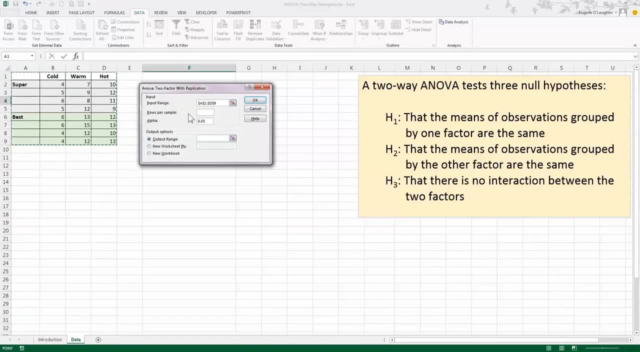 null values in Excel. You must have the same number of rows per sample as well. So select everything, including the label. So that's A1 to D9 in my case. here Our second input box here is: we must tell Excel how many rows per sample there are. So if we look at our data we can see that 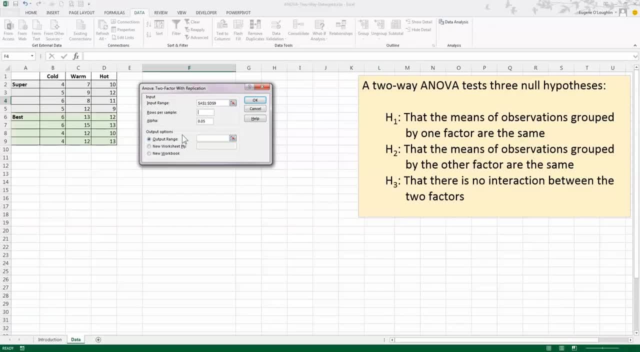 there are four rows for super and four rows for best. Again, these must be the same, So I'm going to type in four here. Our third input value here is our alpha value that we want to use to test. The default is 0.05.. I'm going to leave it at that, because that's a perfectly acceptable level of. 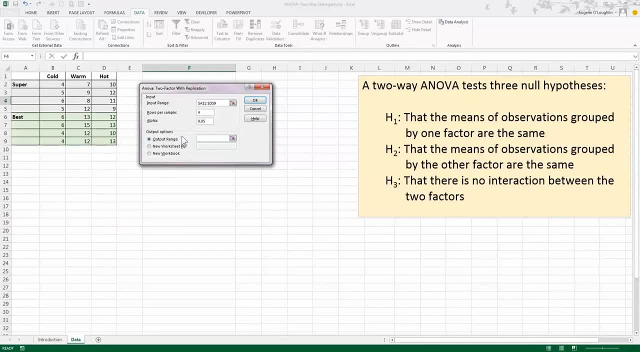 significance to conduct a test of this type. And finally, I want to display my output on the same sheet here. So I'm going to select my output range- Check the output range box here in the middle, and I'm going to select cell F2 to put my output and display it And then click on OK. 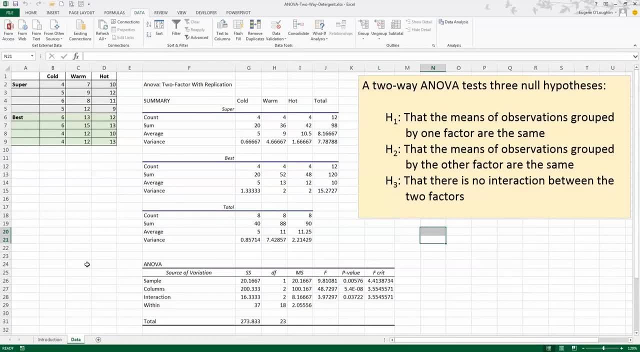 Now this gives me quite a lot of output here. Before I look at the ANOVA table down at the end, let's quickly look at our other data. Excel gives us a lot of summary data. So for the super, it's giving me the count, the sum, the average and the variance for the super brand at each of. 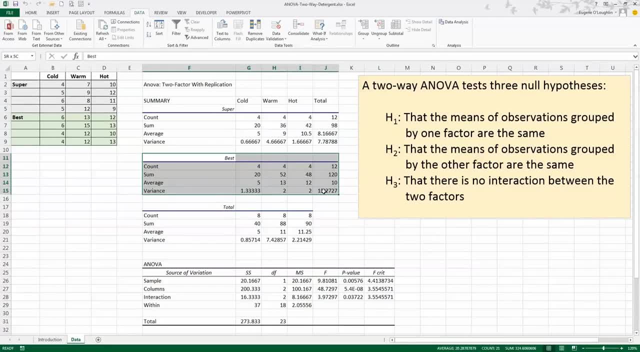 the three temperatures. It's also giving me the descriptors for the best brand, and it's also giving me the descriptors for the totals here as well. So this is going to give you a useful information when you are interpreting your data after you've conducted the two-way ANOVA. 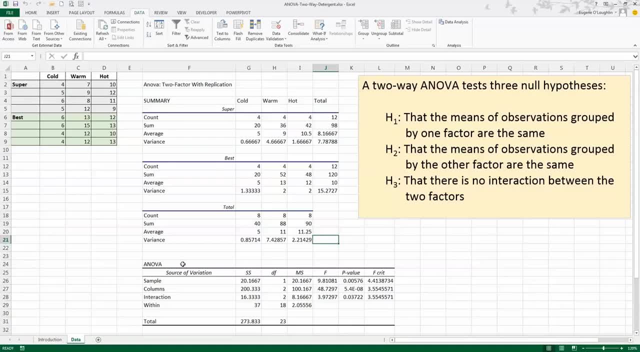 Now the important table is the ANOVA table, down here at the bottom of the screen. It tells us our source of variation. It tells us SS, or sum of squares, the number of degrees of freedom. MS stands for mean square. F is our F or Fisher statistic, which we're looking to calculate. 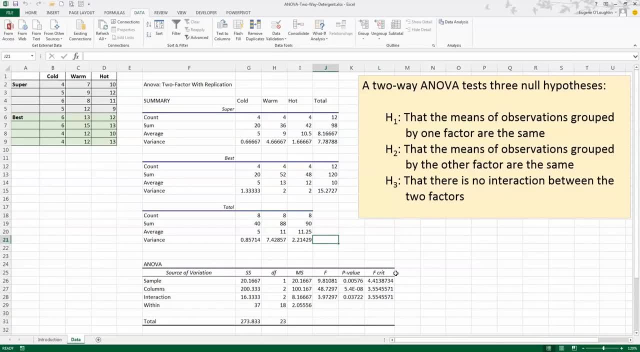 our P value, here is our probability and finally, the F crit is the critical value in the F distribution that will help us decide whether we accept or reject the hypothesis that we have on our screen here. So first of all, let's examine the ANOVA table, and let's look at the first row. 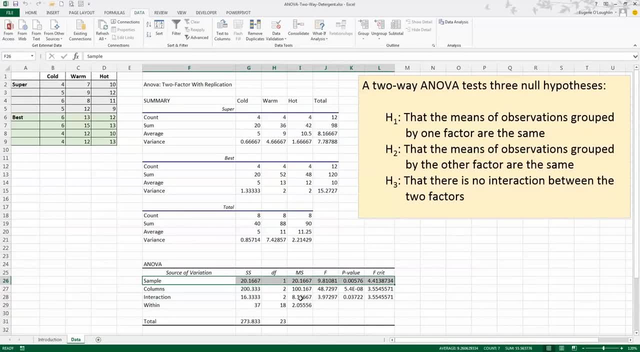 here, which is called the sample row in Excel, and this row here tells us our F statistic and our P value for the differences between the super and best brand here. If you get these confused sometimes the degrees of freedom here is a clue. Degrees of freedom are always the number of 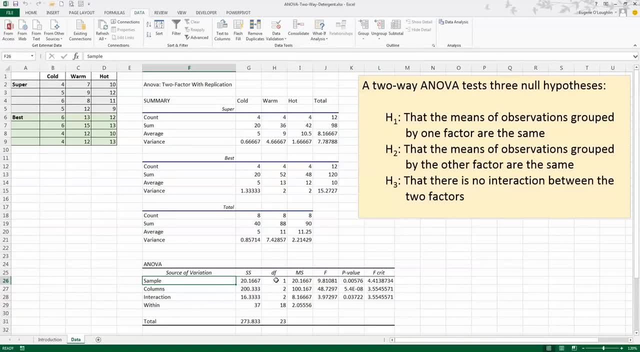 samples minus one. so with super and brand that's two minus one. so we've got one degree of freedom here. The first statistic we're going to look at is the F statistic. We can see it's 9.81 and that's greater than the critical value for this F statistic. therefore, we reject the null hypothesis. 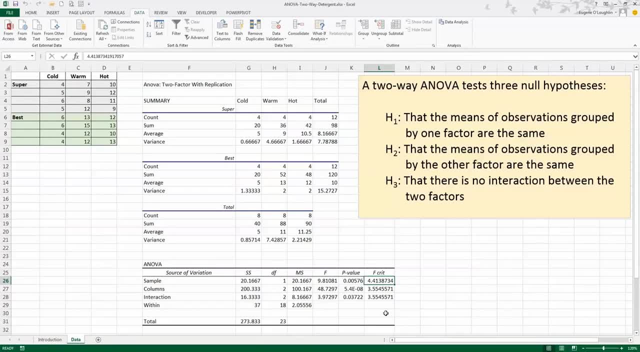 because the means of the observations for the super and best factors are the same, in favour of the alternative hypothesis that they are different. We can also see that our P value here is very small, less than alpha 0.05, which is another evidence for rejecting the null hypothesis. Then we move. 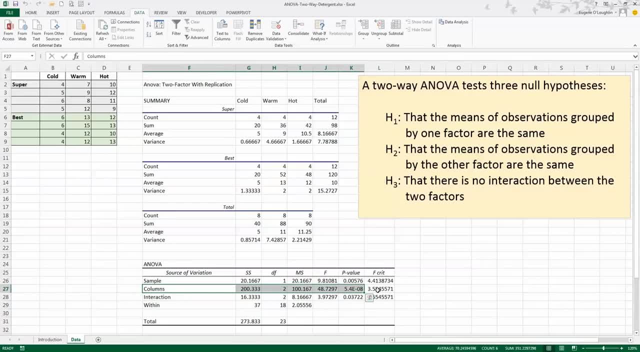 to our columns, which is: is there a difference between the cold, warm and hot values? We can see a very high F statistic here, which is way bigger than our critical value. so 48.7 is our F. Our critical value is only 3.55. therefore, we once again reject a null hypothesis, this time H2. 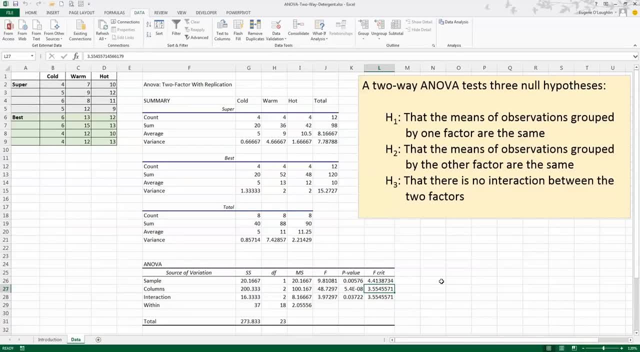 that the means of the observation by the columns- cold, warm and hot here are the same- in favour of the alternative is that there's a difference between at least two of them, and we can also see here our P value is tiny, which is also evidence that we should reject H2.. Finally, we 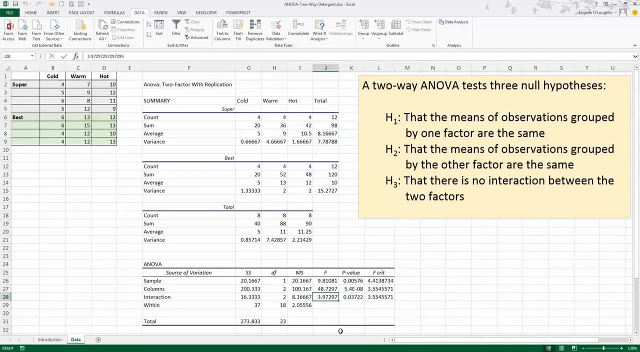 come to our interaction here, and we can see that our F statistic is 3.97, that this is greater than our F critical value of 3.55, and this, of course, is set at alpha equal to 0.05. therefore, even though it's only marginally higher than our critical value, we must reject the null hypothesis that 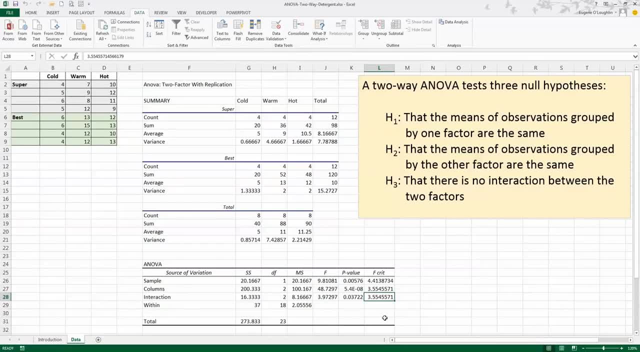 there is no interaction between the two factors, in favour of the alternative hypothesis that there is an interaction. We can also see that our P value here is less than our alpha value of 0.05, so we also will reject in that instance and what this tells us here in the with the interaction is it. 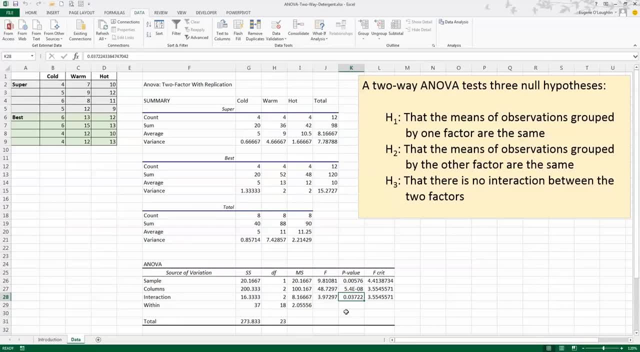 tells us that the effect of temperature on the amount of dirt removed is dependent on the brand. It also tells us the reverse here, which is that the effect of the brand on the amount of dirt removed is dependent on temperature. So that's how you perform a two-way ANOVA in Excel. I hope you found this video useful. thank you for your attention.